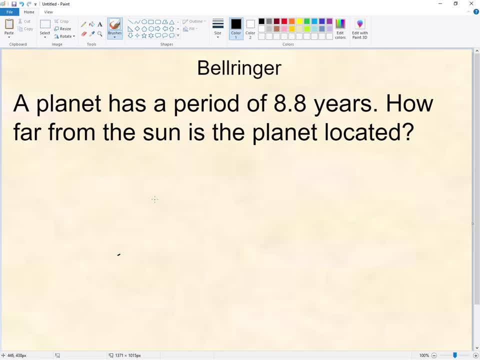 bell ringer pretty quickly here. This is again just Kepler's third law: p squared equals r cubed. So in this scenario we know the period is 8.8 years, so I'm trying to find r. So again, what I prefer to do is just go ahead and symbolically get r by itself. 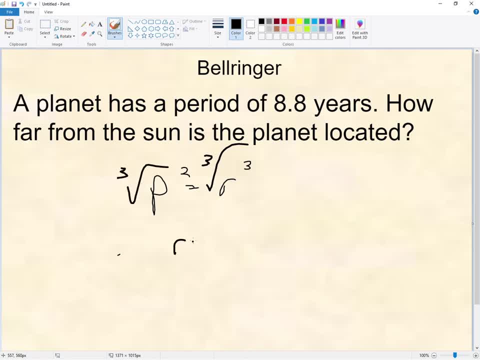 first. So take the cube root of both sides and you have r equals. like I've done several times, this would be p to the two-thirds power. So the distance away from the sun is going to be 8.8 to the two-thirds power. 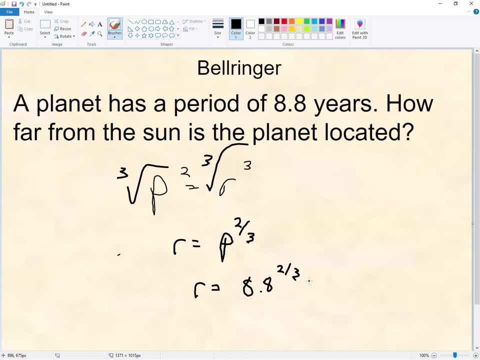 And then just put that into your calculator. We're going to use your calculator a lot today, so if you don't have it out, you may want to get it out, because the numbers we're putting in are pretty big. 8.8 to the two-thirds power gives me approximately 4.3, because this is 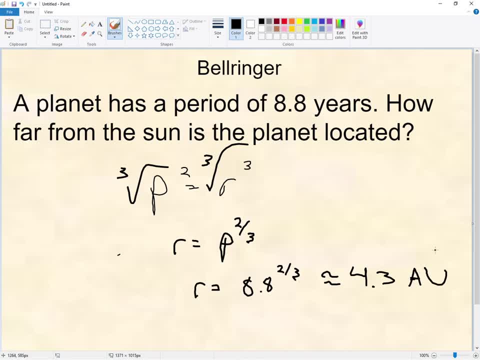 r. this is au, so 4.3 au. So this would be a planet. if a planet had a period of 8.8 years, so it took 8.8 years to go around the sun. one time It's distance would be about 4.3 au, which is about 4.3 times further away from the sun. 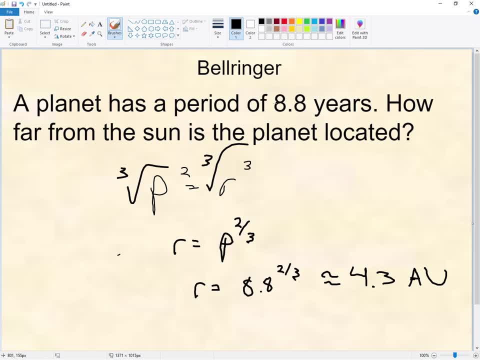 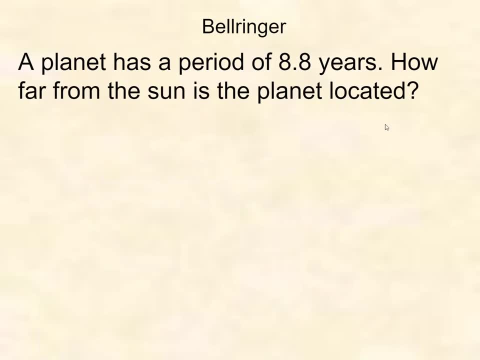 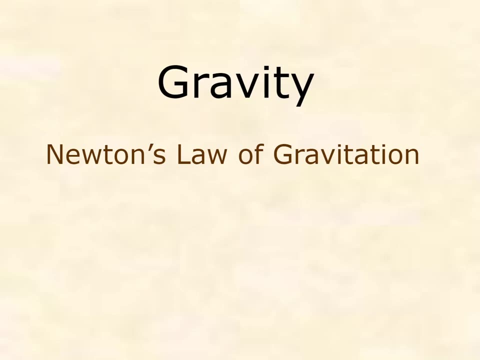 than Earth is, which, again, that at least makes a common-sense check, because if the period's longer, we know it has to be further away. Okay, so, excuse me, we previously talked about Kepler, had established that the planets moved around. 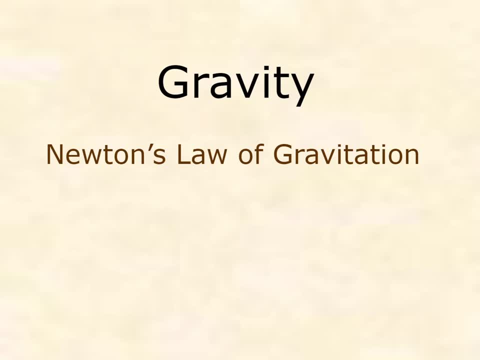 in ellipses. But again, if you were to ask Johannes Kepler, say okay, well, why did they do that? There would be no answer. You don't know. Basically, it's sort of working backwards. This is what a lot of times people do. 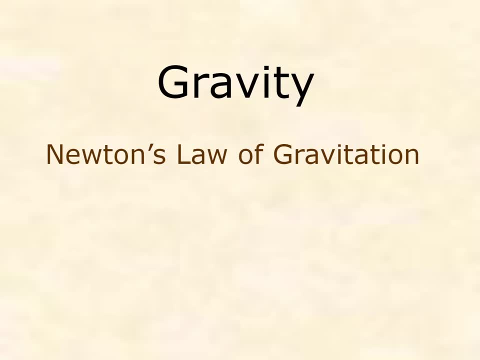 It's almost like guess and check right where you put in an answer and you see if it works out, And if it doesn't, you manipulate your answer until you get what matches your observations. Well, that's what Kepler did, right. 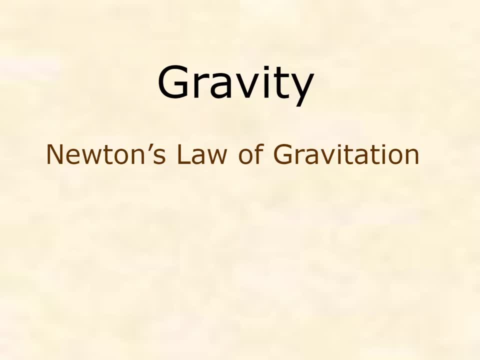 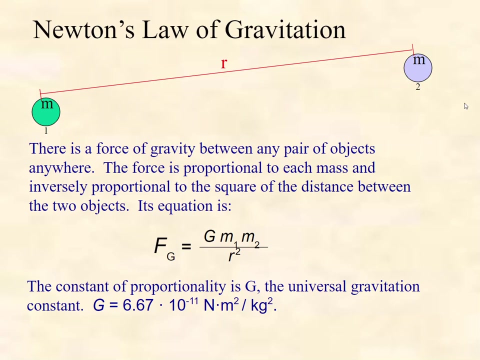 He matched his observations right. He developed a model that matches his observations rather than having a model that predicted observations, so to speak. So he didn't know why. But Isaac Newton don't have a lot of time, unfortunately, to talk about Isaac Newton. 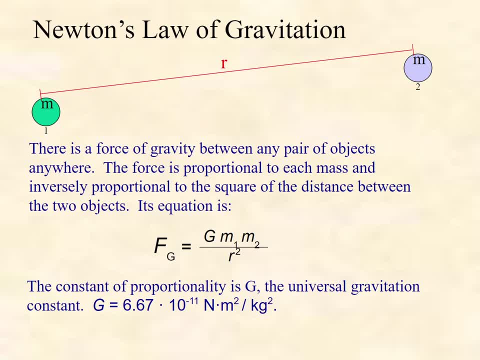 We've talked about him before a little bit, when we talked about Newton's laws. But just genius is an understatement. I mean, he's just a once in a, not even a century. probably once in a century, once in a couple centuries. 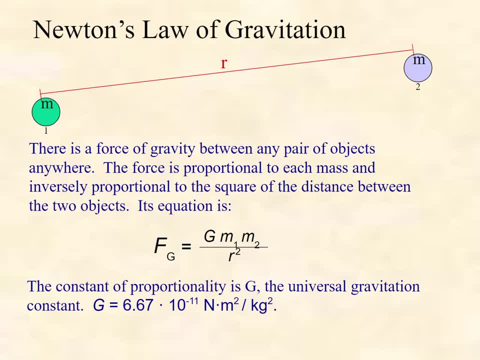 Level of genius: Pretty impressive guy I recently found out. I knew that. if you don't know he well, it's sort of disputed between him and another mathematician named Leibniz who developed calculus, And some people think they both developed it independently. 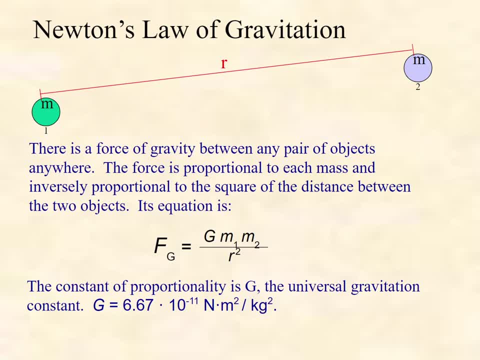 Regardless, Isaac Newton is credited with developing calculus And supposedly he developed it during there was a virus, a disease going around and they had to quarantine. So he, in quarantine, developed it, Or developed calculus, which is pretty impressive stuff. 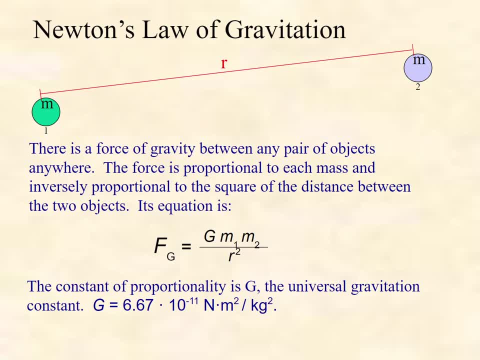 Anyways, one of the things that Newton came up with is his law of gravity. So there's obviously this apocryphal story about Isaac Newton, you know, sitting under a tree and an apple falls on his head, and then he, like, thinks of gravity. 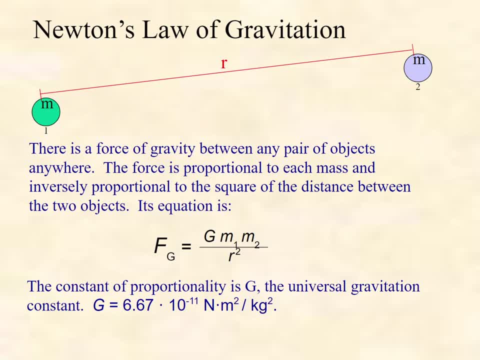 But it's not exactly. Everybody knew that stuff fell to the ground, right? No one was surprised that stuff fell to the ground. But if you were to ask why stuff fell to the ground again, you wouldn't have a good answer. 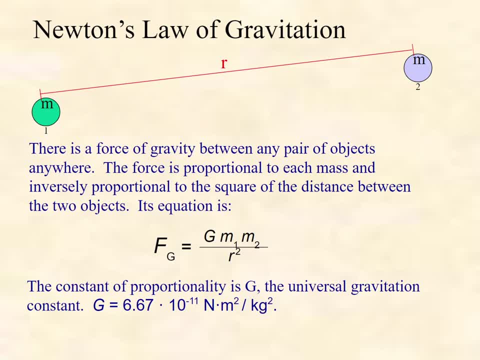 Aristotle had come up with a theory that, you know, things on Earth just fell in straight lines down to the ground, But there was no real reason why Isaac Newton was the first person to put into words what's going on. So, at its core, gravity is simply the attraction that mass has to other mass. 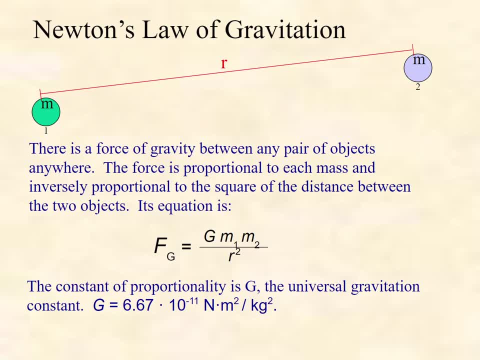 So stuff is attracted together, Stuff that has mass, But this force is very weak. Okay, When we think of gravity, we probably think of gravity like it's a force that's strong or whatever, But it's actually an incredibly weak force. 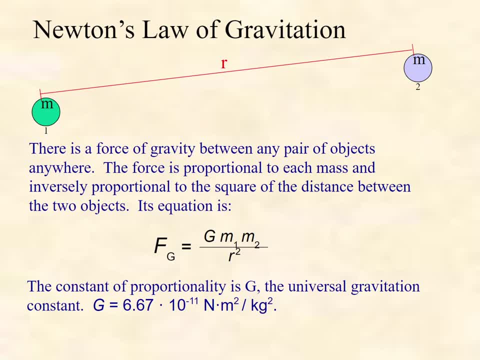 It's the weakest of the four forces that we know of if you look at them in direct magnitude, But gravity works over long distances And gravity becomes noticeable when you have something that's very large, Right? So think about the Earth, right? 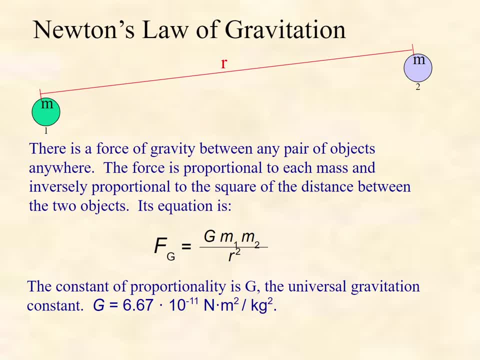 The Earth is huge, All of its mass right, All of the mass that makes up Earth, every bit is pulling right now on. for example, I have a calculator on my desk. It's pulling on this calculator, This entire object right. 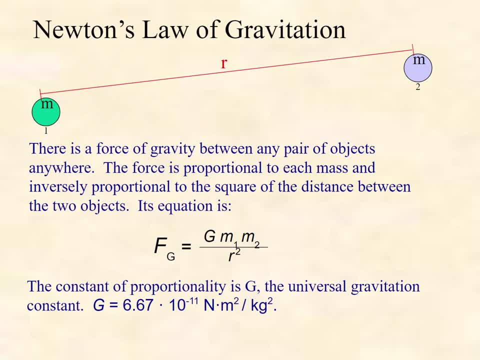 Earth is bigger than you can ever see. You can spend your whole lifetime trying to see all of Earth, And that's just the surface. You're not going to see all of the surface And there's so much more to Earth inside. The point is, the Earth is unimaginably big. 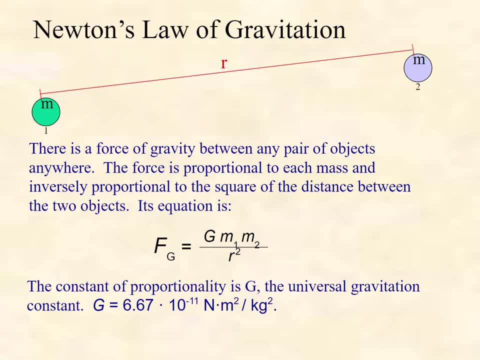 And all of Earth is pulling down the calculator And then I can just pick it up like it's nothing. I just overcame all of Earth's gravity working on this calculator by picking it up. Even something relatively heavy people can pick up. 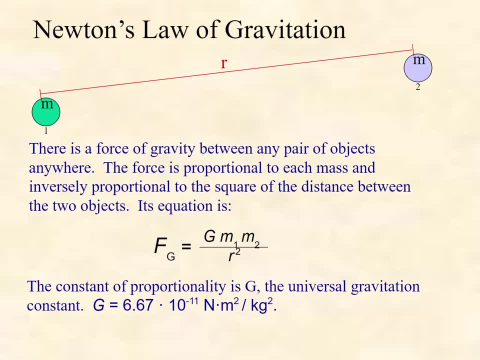 Right. We're able to overcome the entire Earth's gravity simply with our- you know, human muscles. Gravity is incredibly weak, even on a big scale, But it does work over larger distances better than other fundamental forces. So what you see here, this equation, this is Newton's law of gravitation. 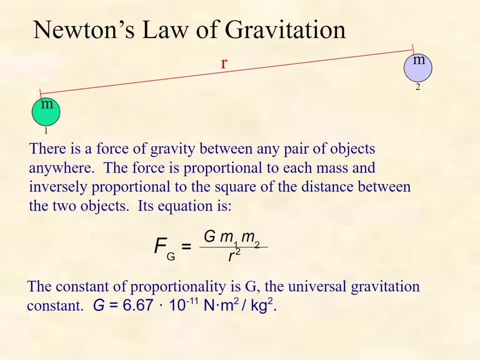 And so obviously you've got this PowerPoint here. access this PowerPoint. We're going to use this equation several times, So you only need to have this. You have here Fg- This is the force of gravity- is going to be equal to. 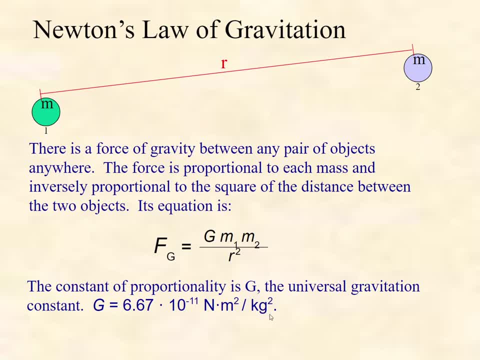 This big G. This is called the universal gravitational constant. It's just a number. It's a number that what these constants do is they work with the units. They make sure that all units work out And they also make sure the units work together in creating this force. 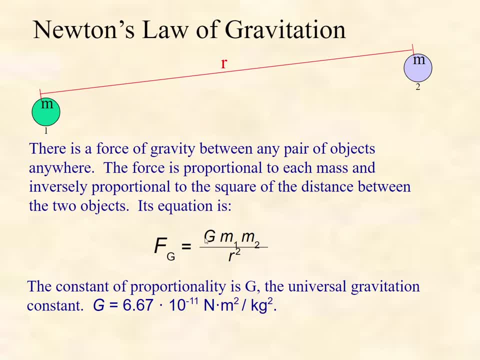 So the constant here. it's important that you have it, But it has no effect. It doesn't change the units, It makes sure everything works out. So you'll have Newton's over here, because it's a force, And Newton's over here. 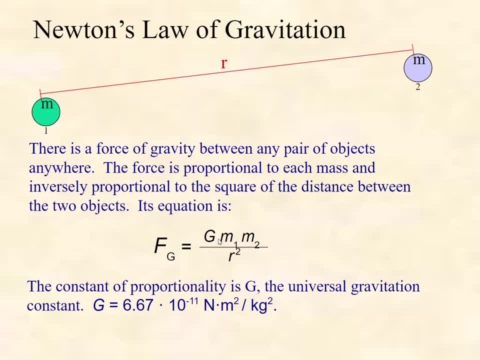 Because it's a force at the end of it. Anyway, so you have big G is the gravitational constant, M is the mass, M2 is the second mass right Because again, it's the force between two masses. So you're going to have both those masses on top and then divided by the distance squared. 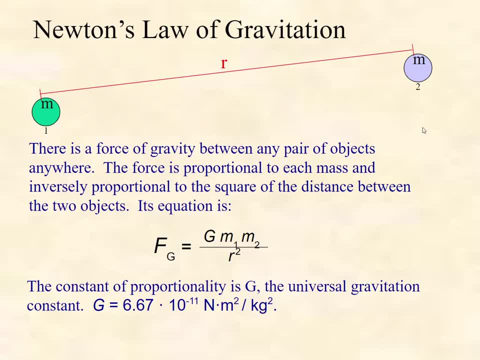 R is the distance between the two. Now this is important. when we have large objects, We are. we are going to use a model where we're assuming That that object is being represented by some infinitely small point with that mass right? So you're going to see this in one of the problems when we talk about Earth, right? 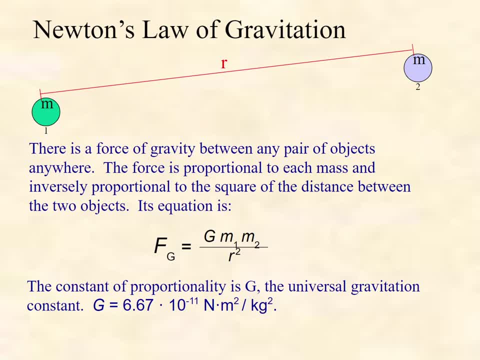 All of Earth is pulling on you. The way that we'll do this calculation is: we're going to assume Earth is one infinitely small point with the mass of Earth And if you're standing on the surface, right you're that, you're the, whatever the radius of the Earth is. 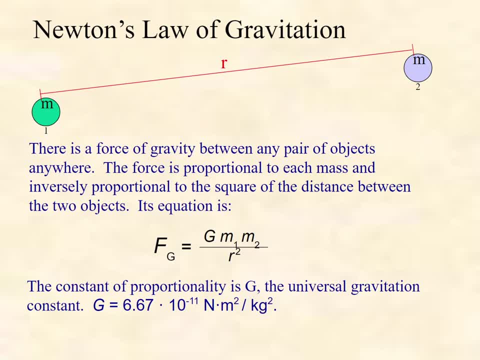 That's how far you are away from Earth, so to speak, And I think you'll see that. OK, so one more time. F is your force of gravity. This is going to be measured in newtons. G is this constant, six point six, seven times ten to the negative eleven. 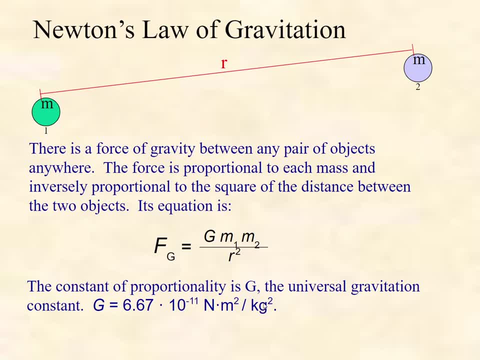 Again, you can ignore this stuff here. This is just the units. I mean, I wouldn't say ignore it, but you don't have to do any, like you don't have to square anything or divide anything. It's just units, right here. 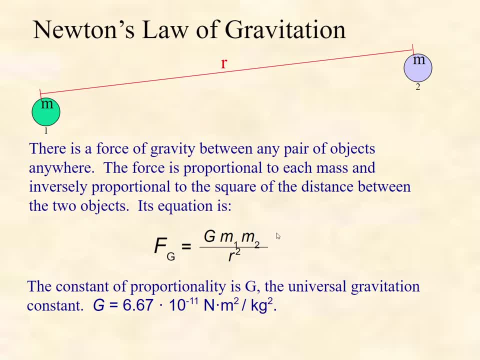 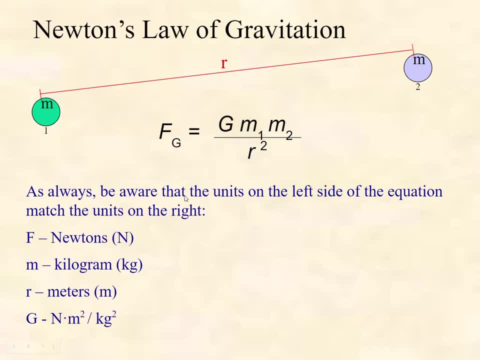 M is the mass of the first object, M2 is the mass of the second object and divided by the distance squared. OK, so you can see some units there And you can see that The units will work out to be the same at the end of this. 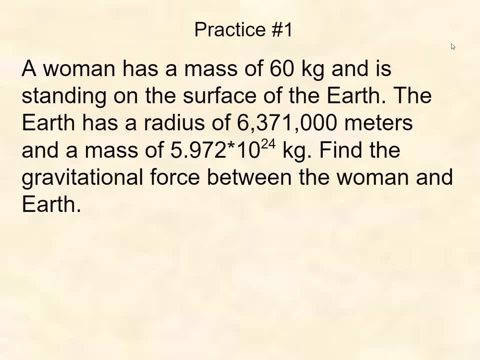 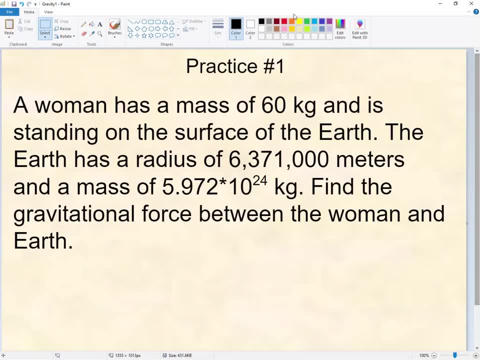 All right, let's look at a practice problem together. We'll do this one together. It says: Let me pull it up over here. A woman has a mass of 60 kilograms and is standing on the surface of Earth. The Earth has a radius of six million three hundred and seventy one thousand meters and a mass of five point nine, seven, two times ten to twenty fourth kilograms. 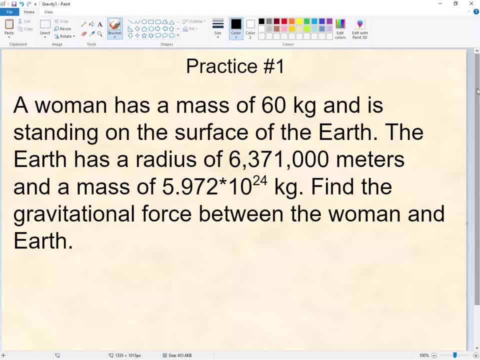 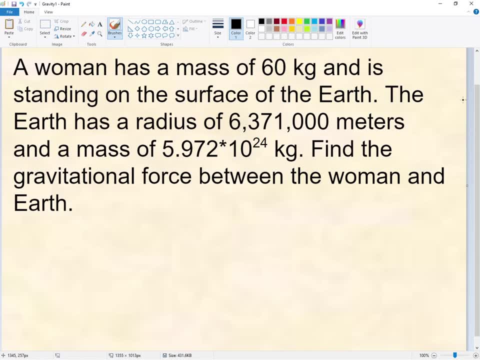 Find the gravitational force between The woman and Earth, All right. So what you need to know is that you know some of these numbers. they'll be big numbers, right. It might look a little ugly, but your final answer shouldn't be too bad. 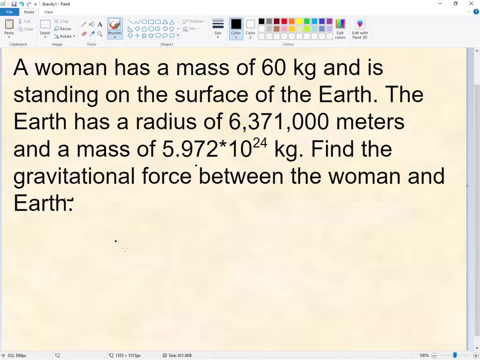 It's just going to be, you know, putting all into the equation. So let's look at this. So I'm going to start by writing my equation. Rewriting: Force of gravity is going to be equal to G times M1 times M2 divided by R squared. 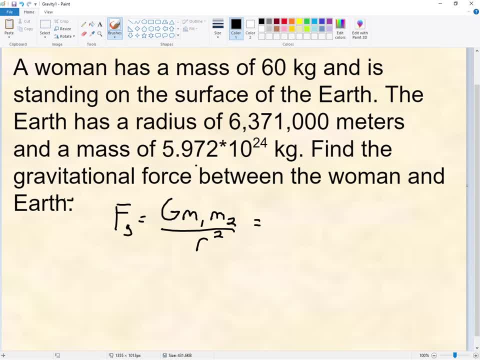 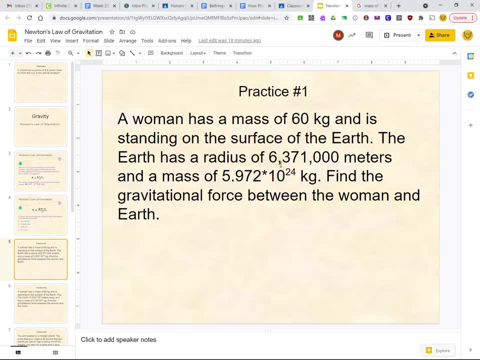 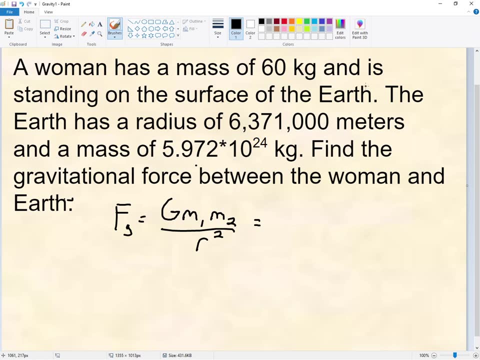 OK, so this is going to be. G is six point six, seven times ten to the negative eleventh. I think. Let me double check that: six point six, point six, seven times ten to the negative eleven. Yeah, So I'm just going to write that up here. 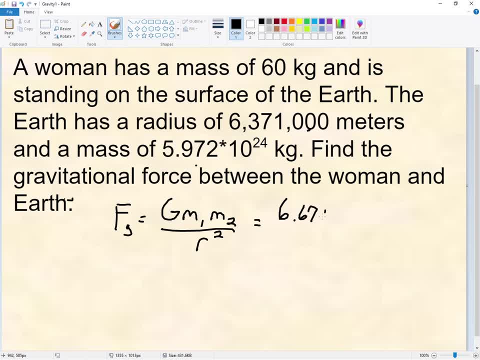 Well, I'll just write here. So G is six point six, seven times ten. to the negative eleven, There's G times. the first mass is the woman And it doesn't matter M1, M2, because it doesn't matter what order you multiply those in. 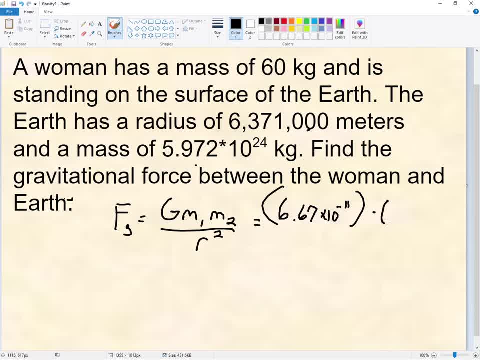 It doesn't matter which one's M1.. It doesn't matter which one's M2.. So times 60 times the mass of the Earth is five point nine, seven, two times ten to the twenty fourth. OK, I'm running out of room already. 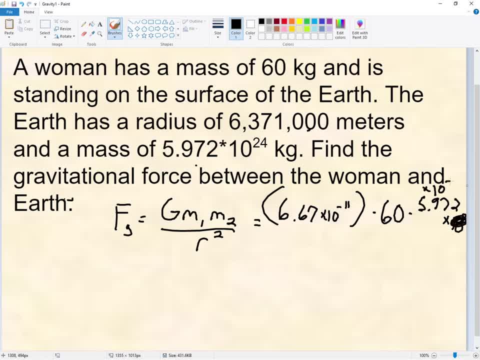 It's not good Times. ten to the twenty fourth, divided by the distance, is Six point three, seven, One times ten to the six. That's just that number in scientific notation. It's that distance squared. OK, so again there's a lot of stuff to put in your calculator here. but it is just calculator work at this point. 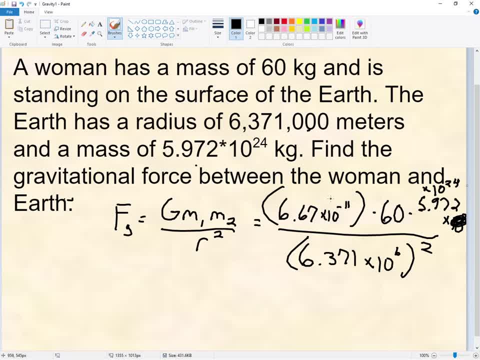 I'm going to do the top. So I'm typing in my calculator: six point six, seven times ten to the negative, eleven Times 60 times five point nine, seven, two times ten to the twenty fourth. OK, so on top. It'd be better if I had this: 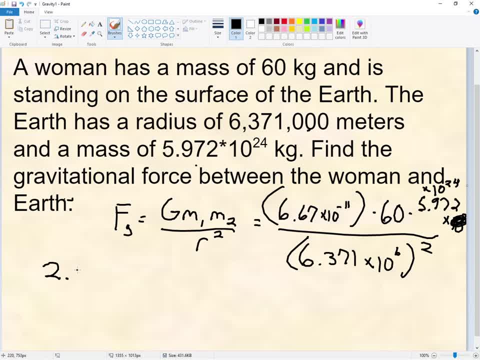 I'll just put in scientific notation. I have two point. OK, just making sure I didn't type in anything incorrectly, because it was smaller than I expected, which is Oh yep, And I did type something incorrectly. I put four instead of twenty four. 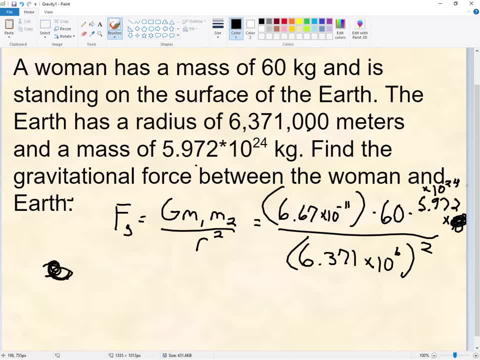 Which would be a pretty big difference. OK, there we go. I knew the number on top of it should get us pretty big. OK, So I get on top. two point: Again, don't worry about rounding too much. Two point three, nine times ten to the sixteenth. 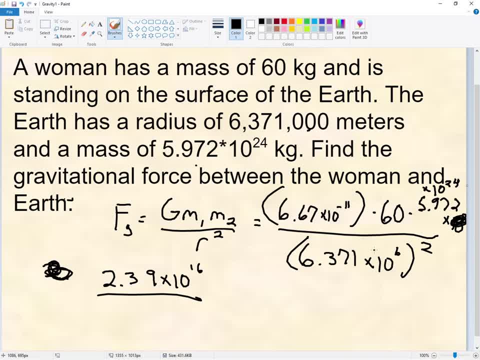 On bottom, if I square this number at six point three, seven one times ten to the sixth. Be careful when you square this in your calculator, Just be sure that you are. I would write it just like I have here, Put in parentheses: six point three, seven one times ten to the sixth. 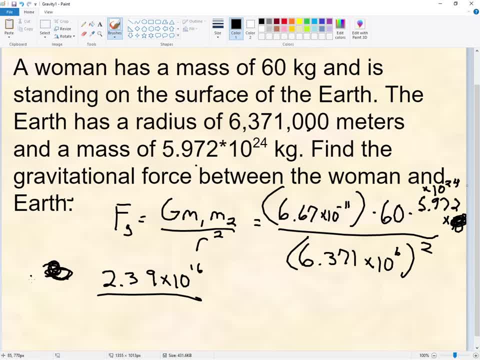 Close parentheses squared. So on the bottom, I get four points, I get four point. We'll just call four point zero, six times ten to the 13th, And then again, be very careful when you divide these. I'm putting. 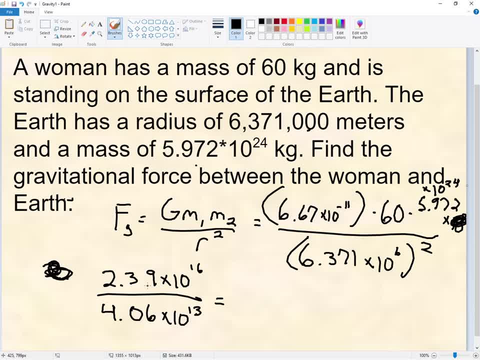 I'm going to say exactly what I'm typing into my calculator. So I'm putting in open parentheses: two point three, nine times ten to the sixteenth, Close parentheses. Divide it by open parentheses: four point zero, six times ten to the 13th. 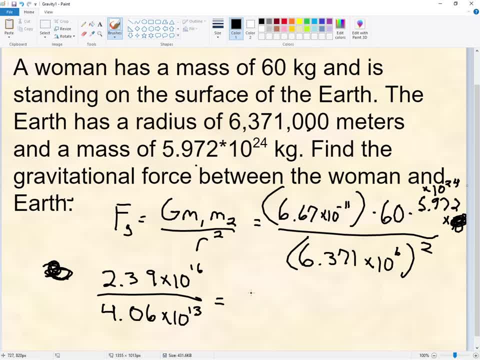 Close parentheses. Okay, so all that and my final answer here is 588.7 newtons. Again, don't worry about rounding too much, but hopefully you're getting around 589,, 590, somewhere around there. So that's the gravitational force. 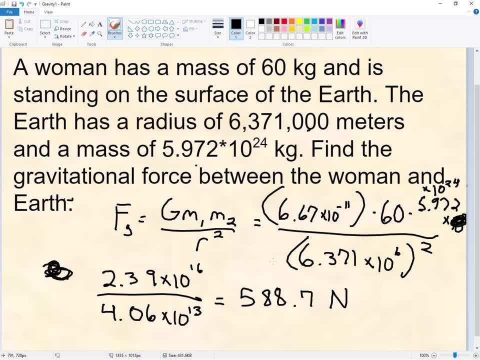 I want to point out real fast: for all objects on Earth, right on Earth's surface, right we can make an approximation, and these things right here. if let's say M1 is the Earth's mass again, then all of these things right here, right for all objects on Earth's surface. 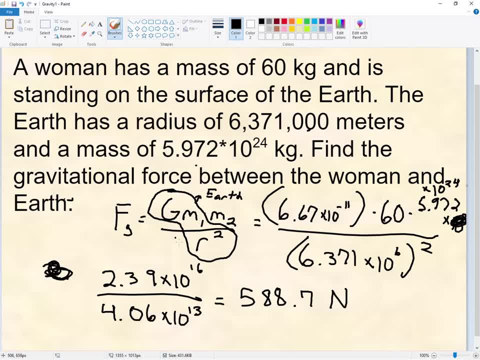 are basically the same. Okay, and I'm not going to do it because, again, I want to have more time for practice. so I'm not going to do the calculation right now. but I'm telling you now, if you put in G times, the mass of the Earth, 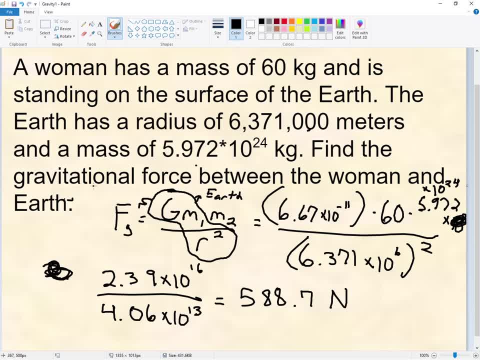 divided by the radius of Earth squared, you should get 9.8.. That's what you should get Because, remember, the force of gravity is the weight and we know weight is mass, your mass, whatever it is times G, M, times G. 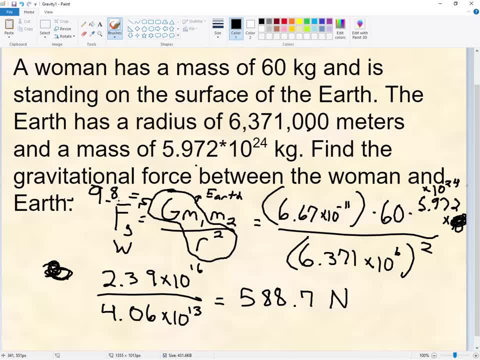 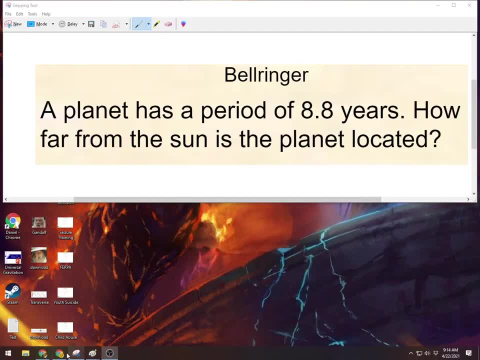 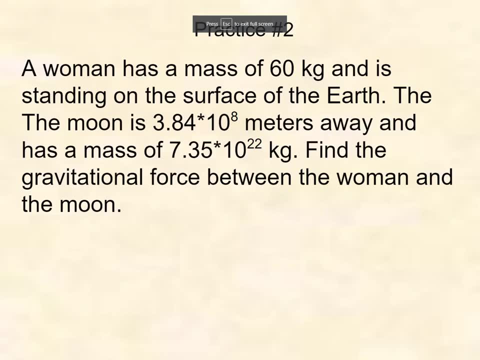 So all this stuff turns into G for Earth, if you're on Earth. Okay, let's look at a second problem. Okay, practice number two. So what I'll encourage you to do is pause. if you're watching the recording, pause it. 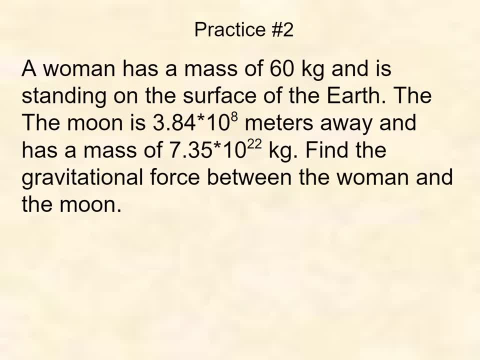 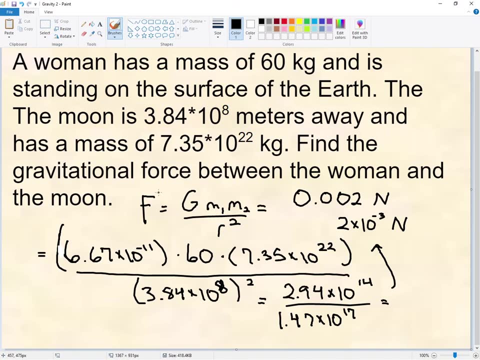 and then, if you're in class live, go ahead and try to calculate this one. This one's maybe a little easier, I don't know, It's the same, really. Okay, here is the answer I got. So, again, just setting up the problem. 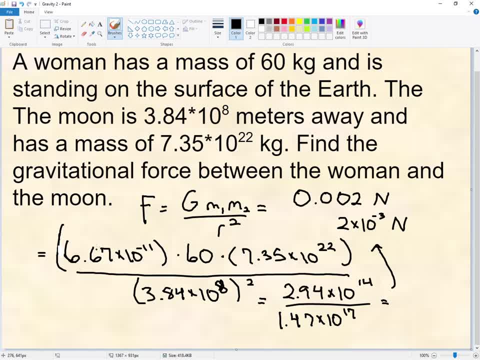 F equals G, M1, M2 divided by R squared G: same thing times. pick one of the masses. again, it doesn't matter which one is which, but 60 is one of the masses times the other mass is the moon's mass divided by the. 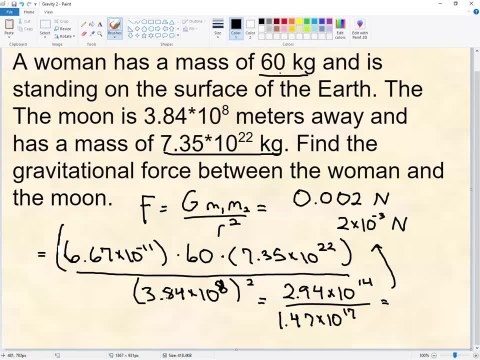 distance squared, there's the distance between them. so again, just like calculator work, on top I punched in and got 2.94 times 10 to the 14th. on the bottom. when I squared that, I got 1.47 times 10 to the 17th. again, just be. 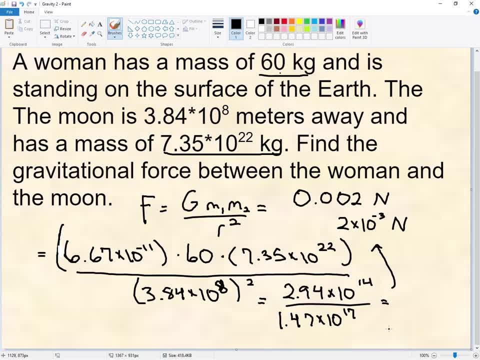 careful by using in parentheses and squaring, and then I got for my final answer: 0.002 newtons, or 2 times 10 to negative third newtons. either way, you want to look at that? so real quick. what does this mean? this is the using, this is the gravitational force that exists between you and the moon. okay, it's not a lot. moon is very far away, so it doesn't exert a lot of force on you. that is to say that you weigh point zero, zero, two newtons less when the moon is above you, right? so? 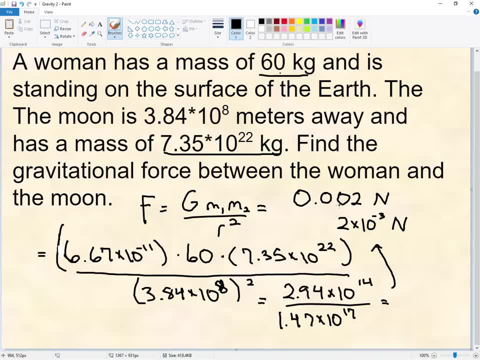 think about, like, if it's a full moon and the moon's right above you would weigh that much less. likewise, you'd weigh that much more when the moon is directly below you, so your weight could fluctuate by the amount the moon there. now that's not very much, obviously. zeros point zero, two point zero. zero. two newtons is let's. 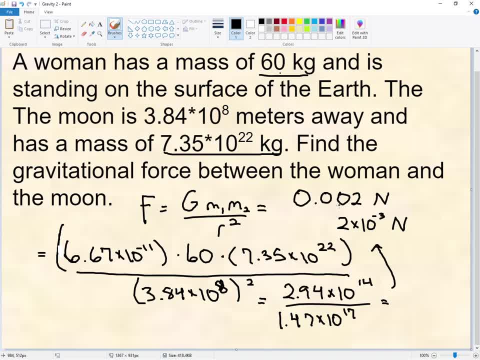 see, go from Newton's and we divide by the nine, point eight, that would be in kilograms. so multiply that by two point two, that's about point zero, zero, zero, four, four, eight, nine pounds. you turn that in ounces about seven hundred seven thousandths of an ounce. so again pretty negligible amounts of force that exists. 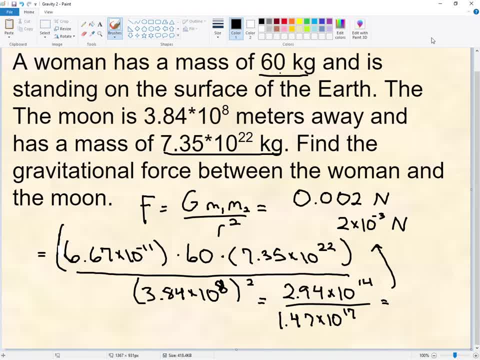 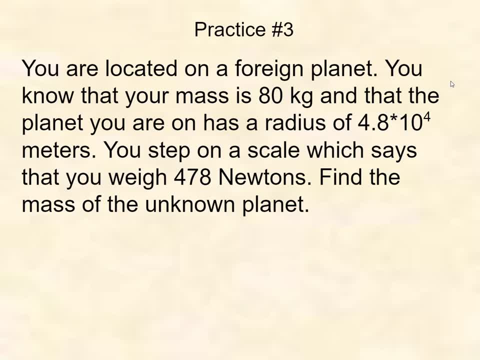 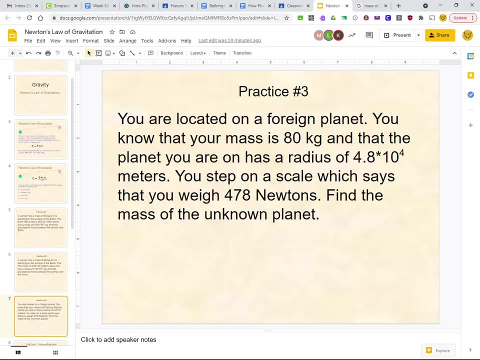 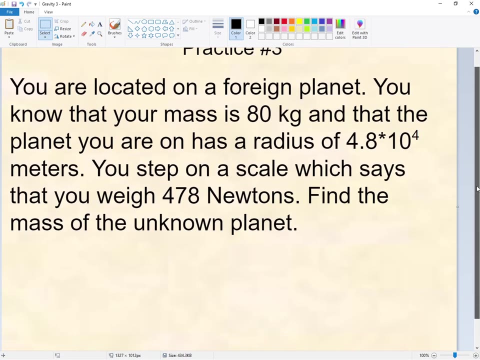 between you and the moon. okay, let's look at another one. this one is a little different, though. we're looking for something else, right? so this time we're looking for a different, a different thing. so let's look at that together. let me pull up my copy of this. all right, here we go. so this is you're. 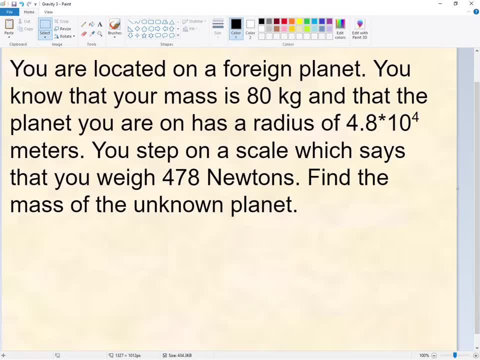 located on a foreign planet. so we don't know what planet this is, some, some other planet. and it says: you know, your mass is eighty kilograms. if the planet you're on has a radius of four point eight times ten to the fourth meters, you step on a. 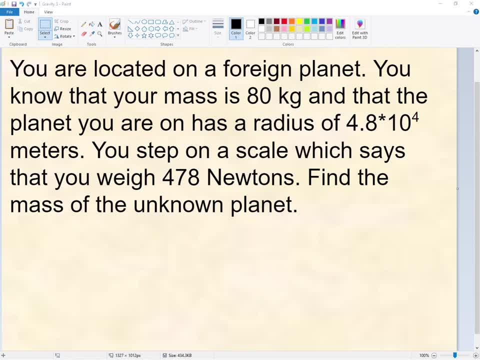 scale which says that you weigh four hundred seventy-eight Newtons, fund the mass of the unknown planet planet. So this time we're not trying to find the gravitational force. We know the gravitational force is 478 newtons. And just to be clear when we say weight and gravitational force, 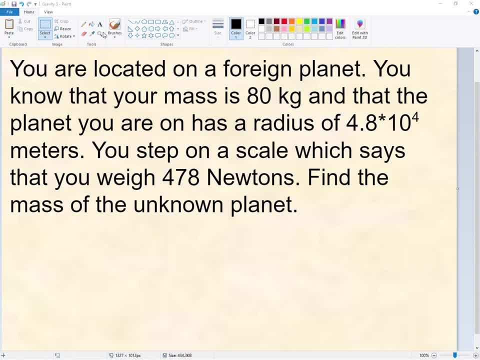 those are the exact same things. That is what the gravitational force means. So let's just write the equation first, and then I'll show you how I would approach this. So the force of gravity is going to be obviously big: G, M1, M2, divided by R, squared. 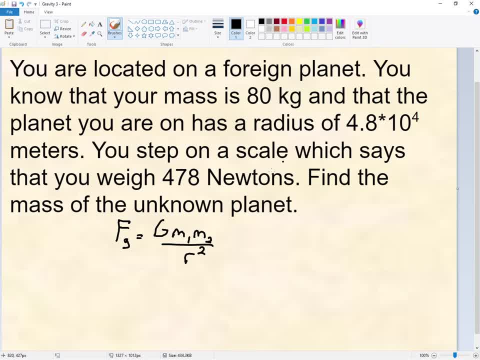 So there are two ways you can do this. Number one: you can put numbers, substitute numbers, into the equation And you'll have everything except one of these masses. Let's just for the sake of this, let's say that this is going to be M2, and that we're going to call the 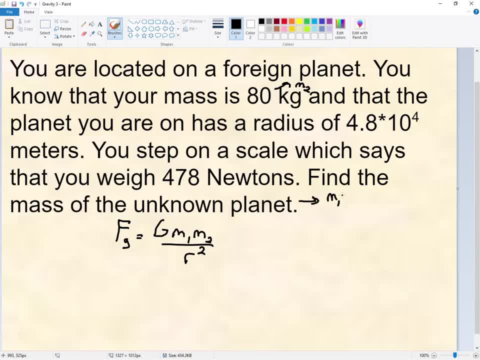 mass of the unknown planet. we're going to call it M1.. Again, it doesn't matter if you switch those up, it won't make a difference. I just want to be consistent here when I'm talking about it, So you'll know all the numbers. 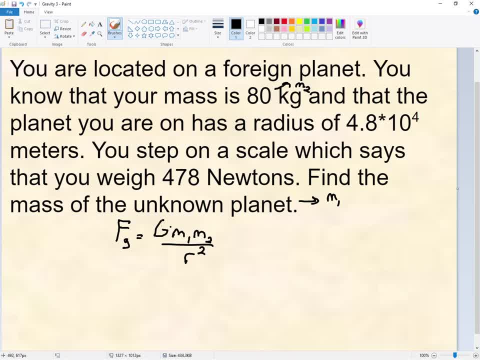 except M1, and then you can, you know, algebraically- move these things around until you get M1 by itself. So you can go ahead and multiply G times M2, you can do R squared, you can divide it and then do that. I think it's actually simpler just to solve it algebraically. 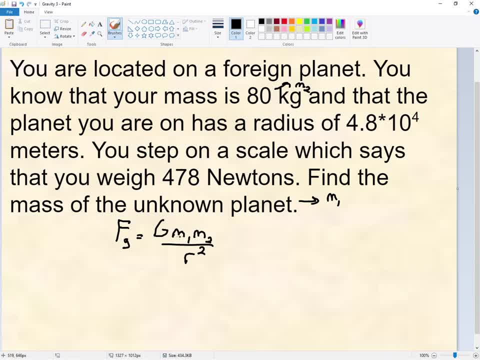 first and then put the numbers in, because then I don't have to worry about doing the numbers calculating and then moving things around. Again, it doesn't matter to me which method you want to use, So I'm just going to go ahead and do that, And then I'm going. 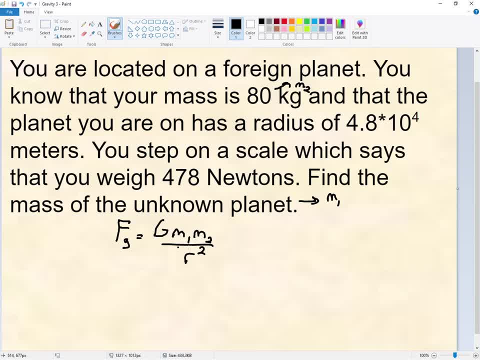 to use, All right. Well, let's say I'm going to do it algebraically first, So I want to get M1 by itself. So what do I need to do to get M1 by itself? First thing I need to do is get rid of G and this M2, okay, Currently I'm multiplying right, I'm taking M1, I'm 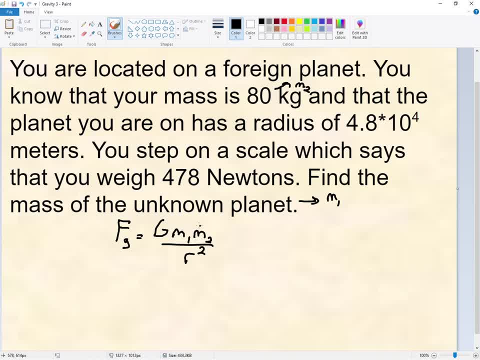 multiplying it by G and I'm multiplying by M2, right. So to get rid of those, I have to do the opposite. The opposite operation of multiplication is division. So I'm going to divide both sides by G and both sides by M2.. 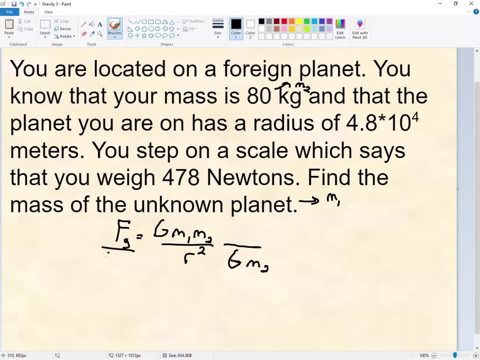 Divide by G. Divide by M2.. Divide by G, Divide by M2.. Okay, Cancels, Cancels, And over here nothing cancels. Then I still have to get rid of this R squared. So right now I'm dividing. 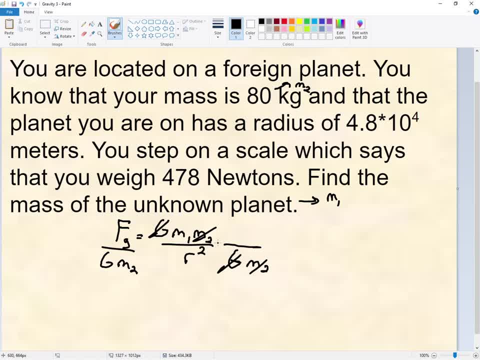 by R squared. So the opposite of division is multiplication. So I multiply both sides by R squared, And again: this side it cancels, This side it doesn't. So now I have this new equation right, So I'm going to rewrite my equation. So on this, 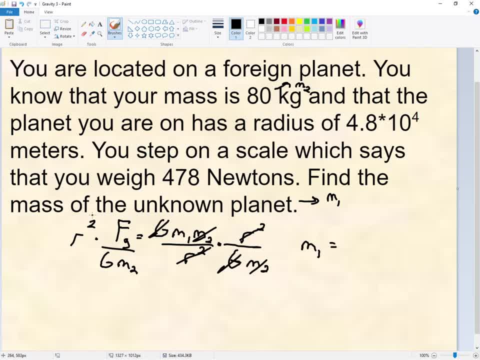 side. I just have M1 equals On the other side. it doesn't matter what order you put these in. I'm just going to put FG first times R squared on top, divided by G times M2 on bottom. Okay, Hopefully that makes sense. Again, all I did was I just did the opposite. 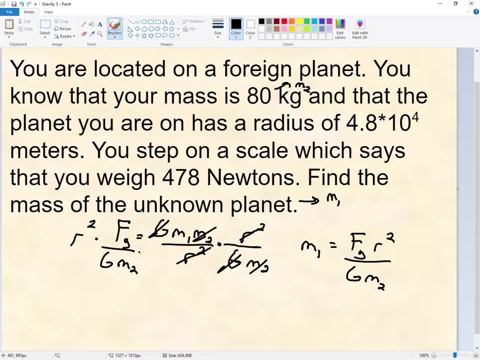 functions of these, to get rid of them on this side, and they went to this other side, Because I have to do the same thing to both sides, And this is my equation. Now again, you don't have to do it this way, But once you have this equation, that's it forever, I mean. 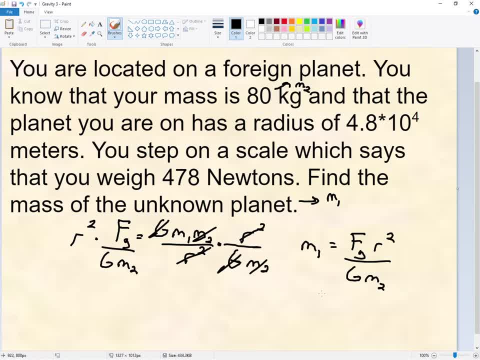 like, since you know, since you can use your notes on the test, you could write this equation down and you have it forever, Like you'll always have it. Okay, So then it's just calculator work. M1 equals The FG is the force of gravity, which we know is newtons, 478 newtons. So 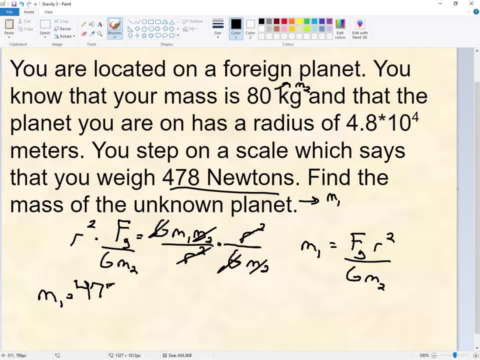 that would be 478.. Times the distance squared, So the distance here is this number, here That's again, that's the distance for the surface. So it's like from the surface to the center. So that's 4.8 times 10 to the fourth, squared divided by G is 6.67 times 10 to the negative 11 times. 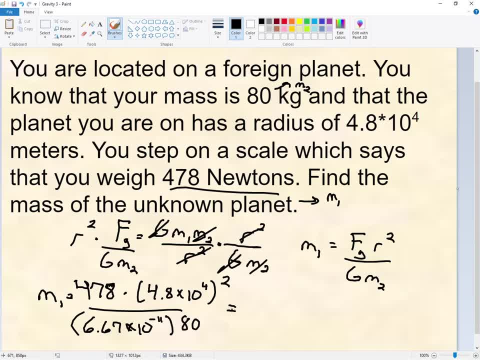 M2 was just 80.. Okay, So again just doing the calculator stuff. I'm going to do 4.8 times 10 to the fourth, in parentheses, squared, and then multiply that by 478.. So on top of this I get 1.1 times. 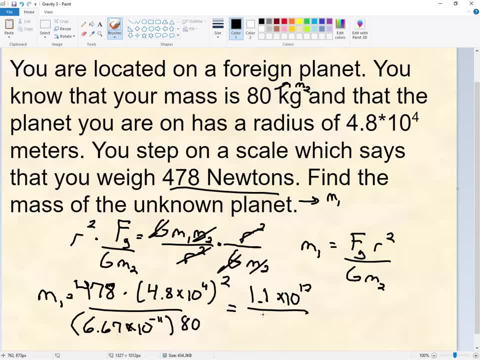 10 to the 12th On bottom. I did 6.67 times 10 to the negative 11. And I got a pretty small number. Let's see if I can get it in scientific mode. There we go. That's 5 times 10 to the negative 9th. Then I just divide, So again I'm doing parentheses. 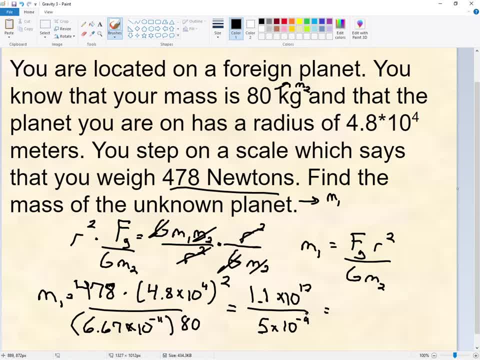 1.1 times 10 to the 12th, Divided by parentheses, 5 times 10 to the negative 9th. So again I'm doing: parentheses 1.1 times 10 to the 12th, Divided by parentheses, 5 times 10 to. 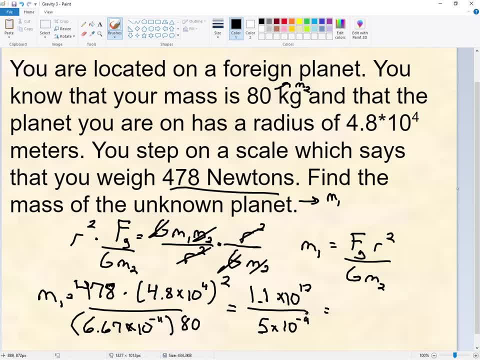 the negative 9th, And for my answer I get 2.2 times 10 to the 20th. This would be kilograms for our mass M1.. Okay, Okay, Okay, Okay, Okay, Okay. Those are all the practice I have. I do want to show you one more thing, though, just so. 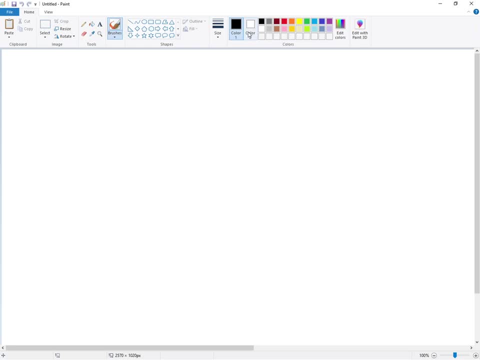 you see it, because I think there is a question like this. Okay, I just want to show you what it looks like if you solve for R, right? So let me rewrite the equation: FG equals big G, M1,, M2, divided by R squared. So what if I wanted to just solve for R squared? So 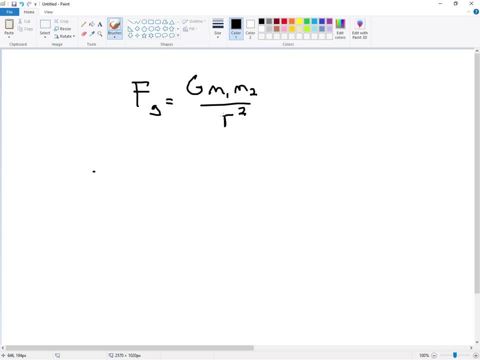 what if I wanted to just solve for R? Like, let's say there's a problem where I knew I wanted a specific force and I wanted to know how far away would I have to be to have that specific force right? So let's say I knew the masses, I knew obviously G and I knew the force and I wanted to find R. So again, I would suggest solving it symbolically first. So if I was trying to get R squared by itself, the first thing I always do if it's in the bottom, get it out of the denominator. So I multiply both sides by R squared. 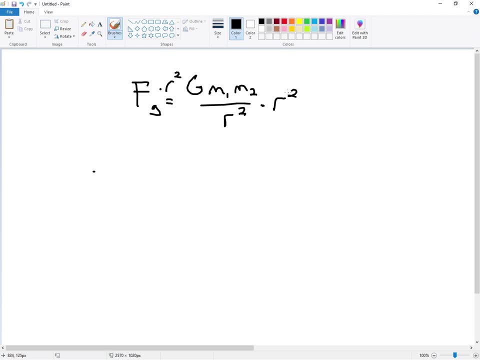 So that it would obviously cancel on this side this little point, and then I would have just R squared. So then I would have F sub G. R squared equals G, M1, M2.. And then if I want to get R by itself, let's get rid of FG first. So I divide both sides by FG.